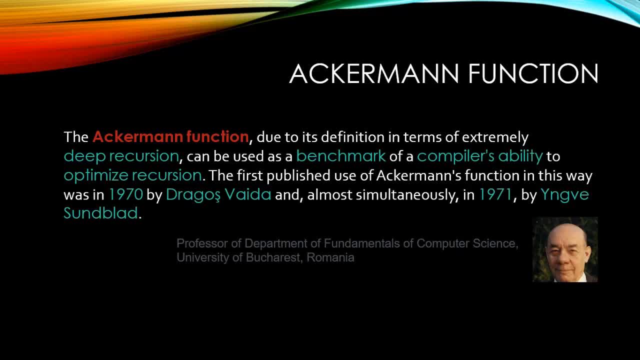 University of Bucharest, Romania, So that is Radios Baida. Okay, another professor from Emeritus of KTH, Chora Institute of Technology, Stockholm, So that is Ingo Sandbladend- Sandbladend, Okay, it's very hard to pronounce the name of that professor. 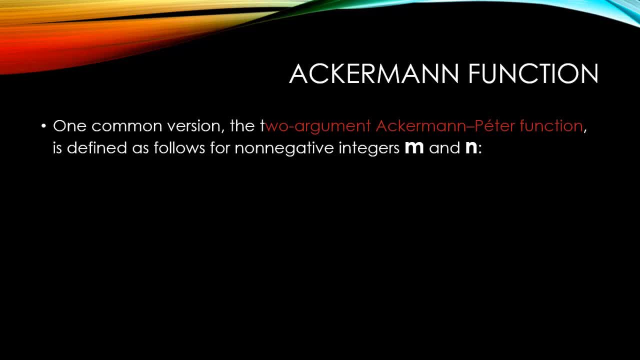 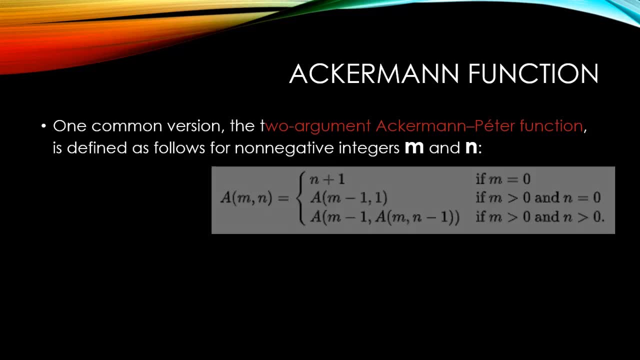 One of the common versions, the two or remote Ackermann-Peter function is defined as values for non-negative integers, m and n. So for m and n we have this formulas. The values from m and n is derived from formula number one, which is if m is equal to zero. 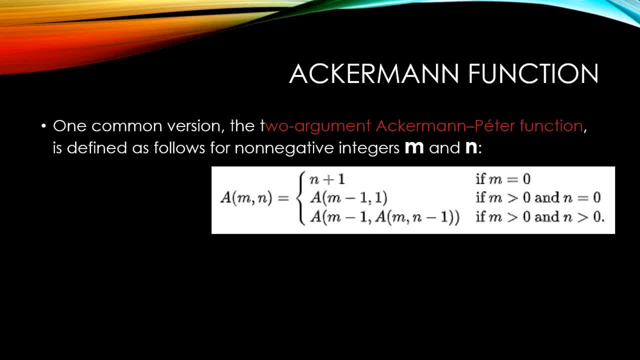 Okay, if m is greater than zero. So that is, the formula would be n minus one comma one. Okay, m is equal to zero. So that means m is equal to zero. So that is the formula would be n minus one comma one. 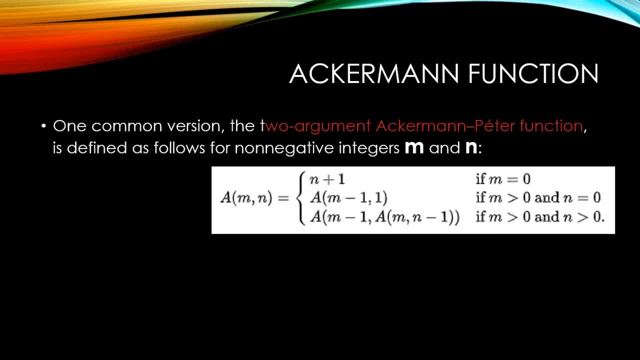 Okay if m is greater than 0 and n is equal to 0, but if m is greater than 0 and n is greater than 0, also the formula, the third formula, is much longer Okay: m minus 1, comma, m comma, n minus 1.. 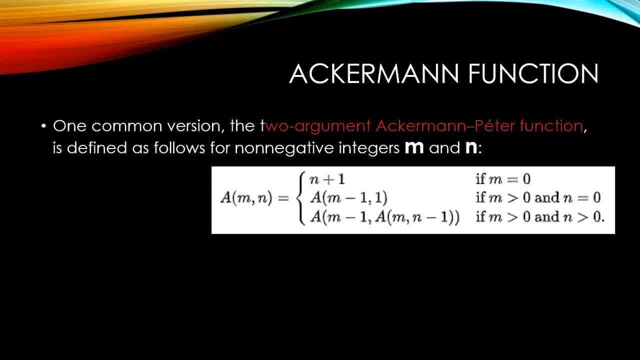 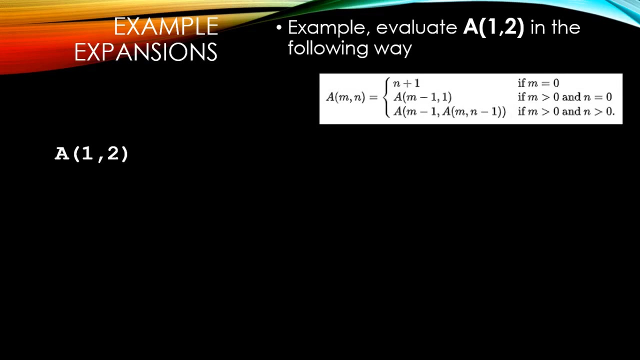 Okay, so that is our third formula, which means if m is greater than 0 and n is greater than 0, the formula will be much more longer, But if m is equal to 0, so the formula is very short. Okay, so we will apply the first example that we have: a command: m is equal to 1, then n is equal to 2.. 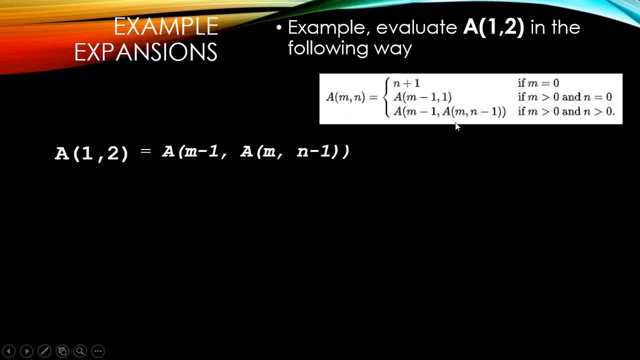 Okay, so if we substitute this in the third formula, so because m and n is greater than 0, so this is d The formula that we will be using If we translate that to m and n. so the values where the values would be okay. 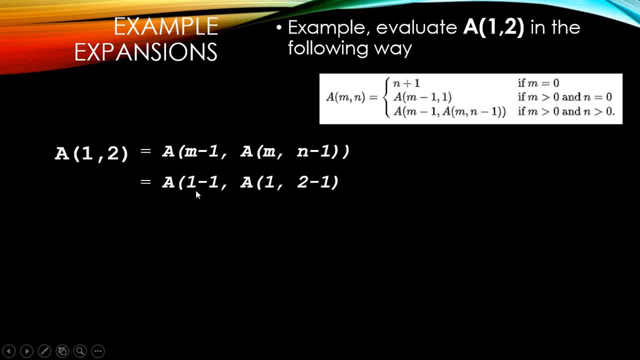 and if we subtract 1 minus 1 here and 2 minus 1 here, so the result would be this one. Okay, then we will evaluate the inner function of this. The inner function of this is a minus, so 1, comma 1, so that would be the third formula. 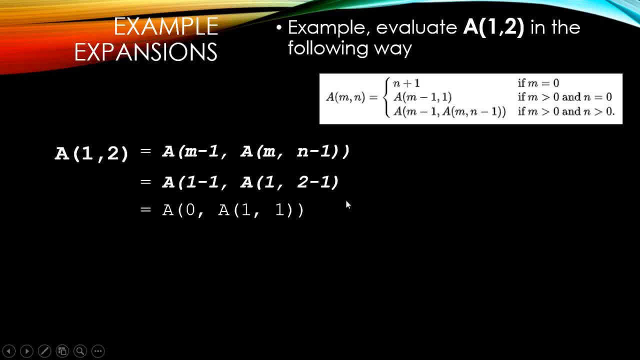 Okay, if m is greater than 1,, bigger than 0, and m is greater than 0, so third formula. Okay, so using this. So all you have to do is translate this to formula number 3.. Okay, so you have this. 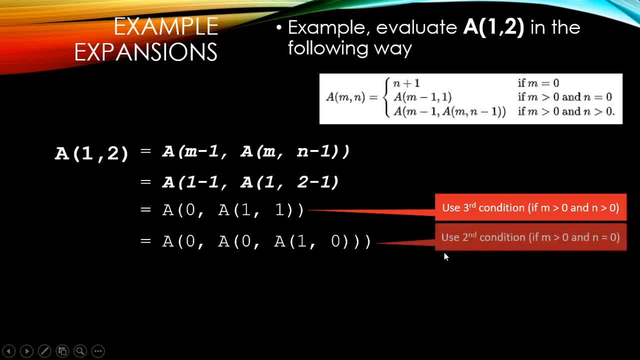 Next is number 2.. Okay, formula number 2, we will apply Because n is 0,, okay, and m is greater than 0, and n is 0. So that's why we will be using m minus 1, comma 1.. 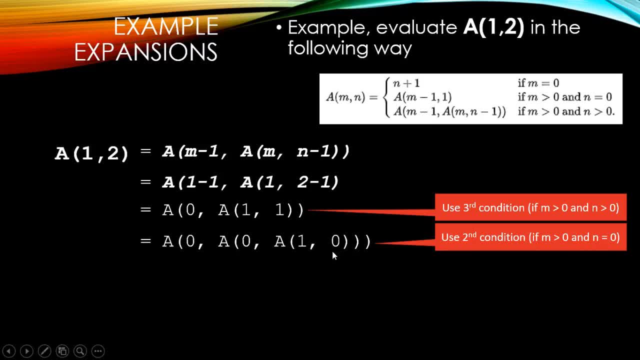 So m minus 1,, so which means this one will become 0, and this one will be 1.. Okay, then next we'll apply the first formula, which is, if m is equal to 0,, then it will be n plus 1, n plus 1.. 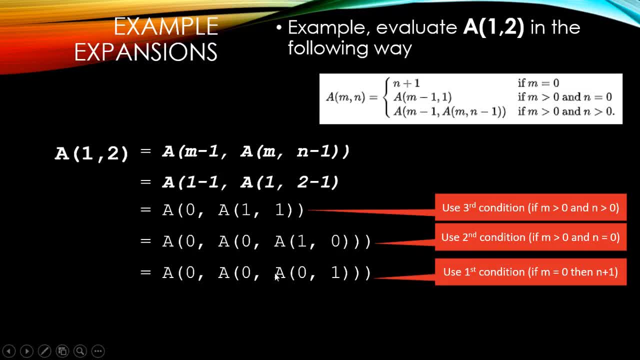 So, which means we will erase. So if m is equal to 0,, then we will replace this one. we will substitute this to 2,. okay, because n plus 1.. So that's why we have 2.. Okay, then again, because m is again 0, then we have 1,, 2,, n. 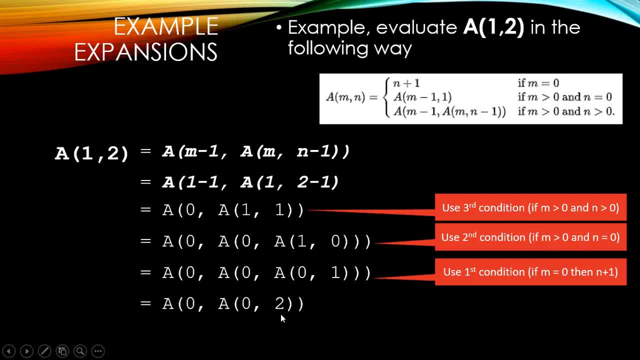 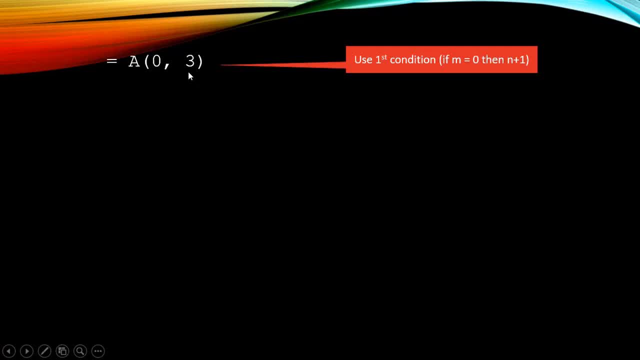 So that's why we will be translating this to number 3, okay, number 3.. Okay, that's it. Then next is formula: again Okay. Then next is formula number 1, okay, because still we have m is 0, okay, so we'll have final answer, which is 4.. 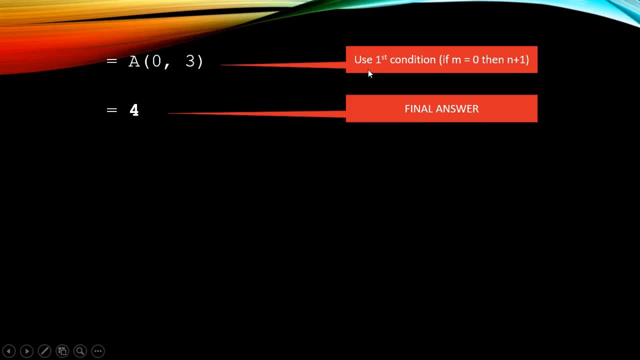 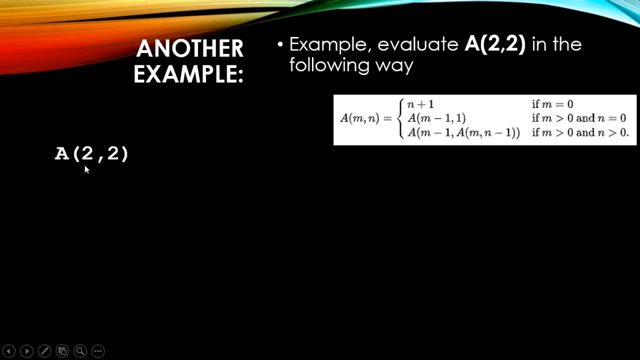 So we'll have n plus 1 for formula number 1, okay, so that's our final answer. Okay, more example: How about if we have m is equal to 2 and n is equal to 2?? So what will happen? 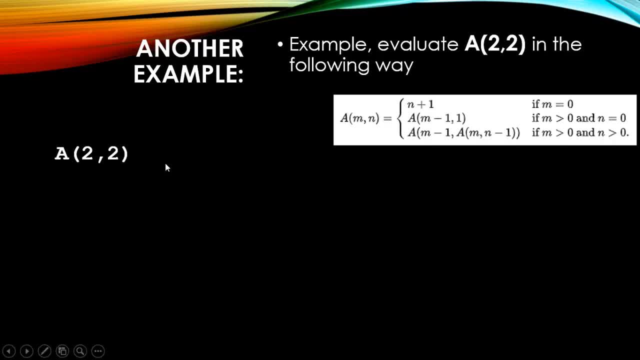 What is the final answer? Okay, so if we try to evaluate this one, so we have to use the third formula again. So in the third formula, we'll be translating this again. As you can see, we have here parenthesis, second parenthesis. 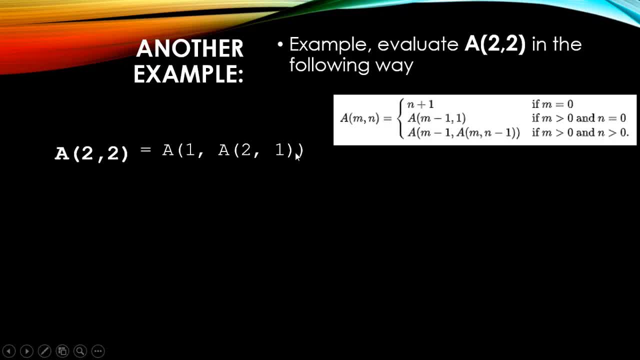 So, whatever opening parenthesis you have, you have 2, close that. Now we have 2, make it equal. You have also 2 closing parenthesis because we have 2 opening parenthesis. So what we have to do is translate this to the third formula, which is m minus 1 comma, m comma, n minus 1, okay. 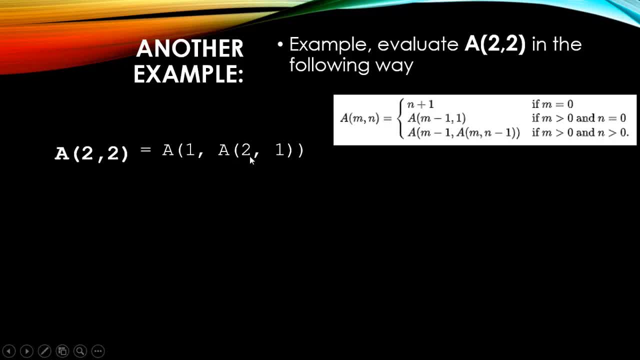 So it will be. it will be more longer, okay? So next we have 2: 0,, 2 0, because this one is 0, the n is 0, so we'll use the second formula, Which is m minus 1 comma 1, so m minus 1 comma 1, okay. 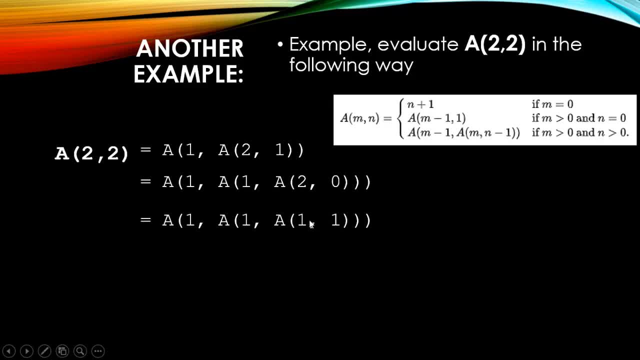 So it will become 1 comma 1, okay. So check, evaluate what is the inner function. So it means we have to concentrate on the inner function. okay, Inner function only. So on the inner function, we have 1 comma 1.. 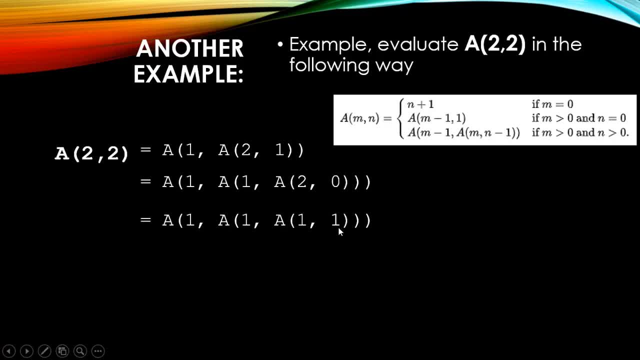 So we will use the third formula again. So it It will be much longer. So if I substitute, it will become this one. okay, Then this one will be substituted to the second formula, okay, Which is m minus 1 comma 1, m minus 1, which will become 0 comma 1, okay. 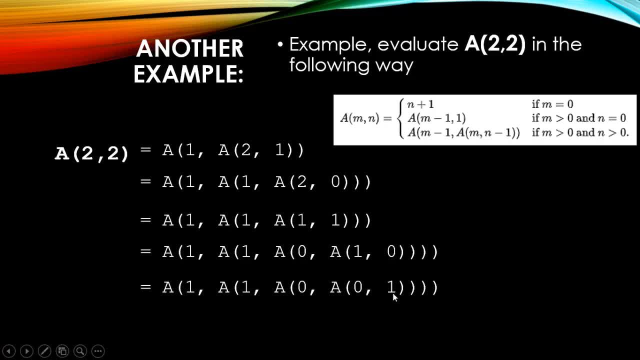 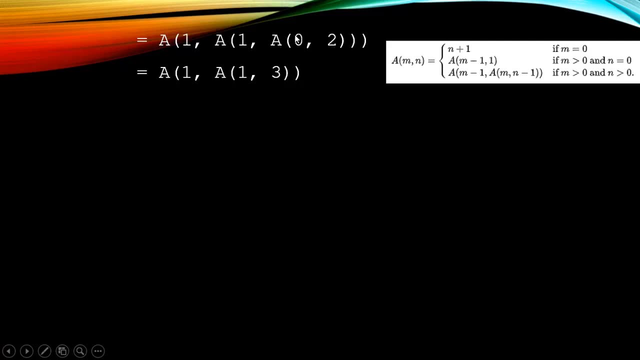 Then here we will use the first formula, which is n plus 1, n plus 1.. So meaning this: This function will become 2, okay, This function will become 2, that's why we have 2.. Then we have again: m is 0, so which means we have to use n plus 1, n plus 1, so we have 3, okay. 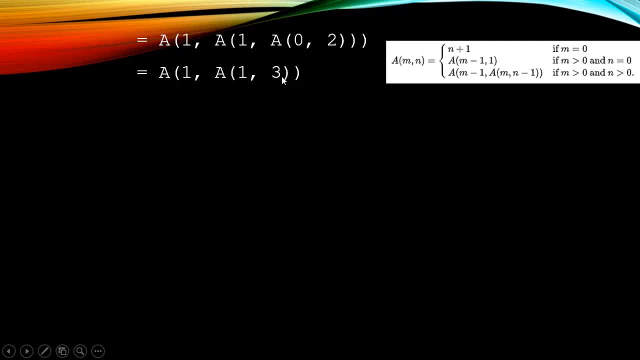 But this time we have n is 1 and n is 3, so which means this is the third formula. okay, And the third formula, So we will have. We will have to translate this again to the Ackermann algorithm, okay. 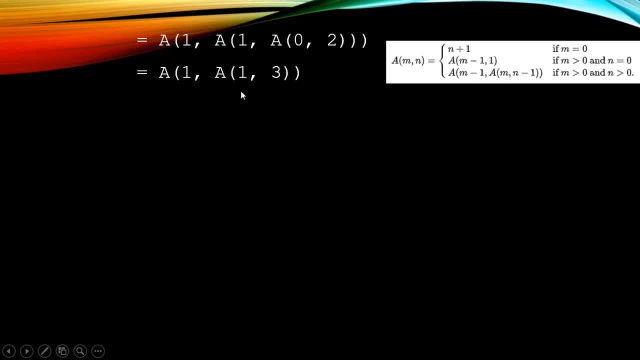 Our Ackermann function here, which is the third formula. okay, So the substitute value would be this one. okay, So again we have 1, 2, so we have to do This is the third formula, so it will be m minus 1 comma, m comma n minus 1, okay. 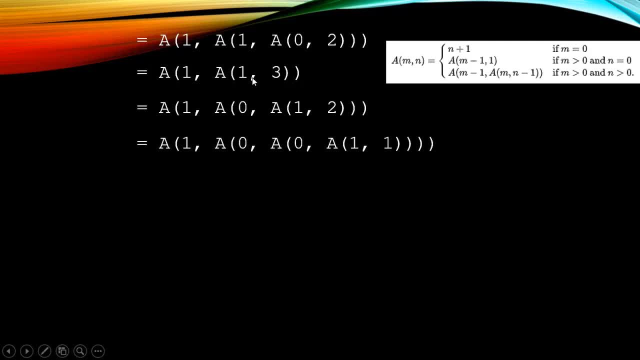 Okay, again, as you can see here the values will become longer and also the formula okay, for our Ackermann function will become longer. Here at the right side of the inner Ackermann function, as you can see, the decreasing order, the decreasing order of the number, is used. okay. 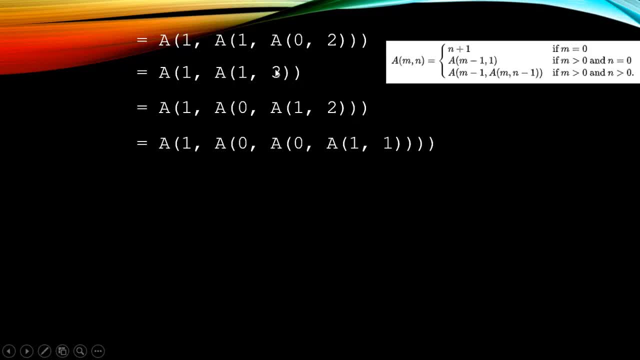 So we have, We have here a proper for our Ackermann algorithm. So again 1, 1,. so it will be the last part: 1, 0, okay. So here we have to use the second formula, which is 0, then 1, okay. 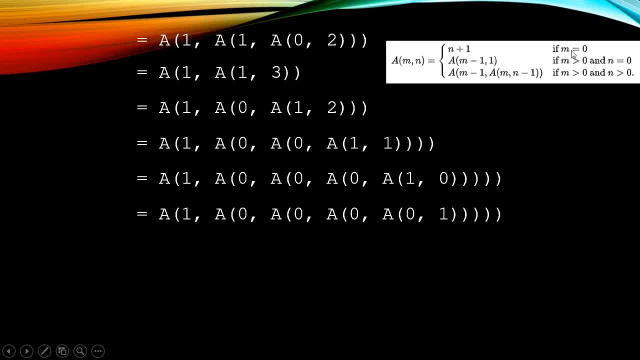